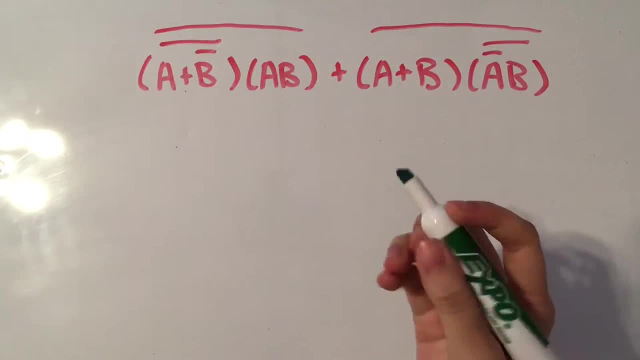 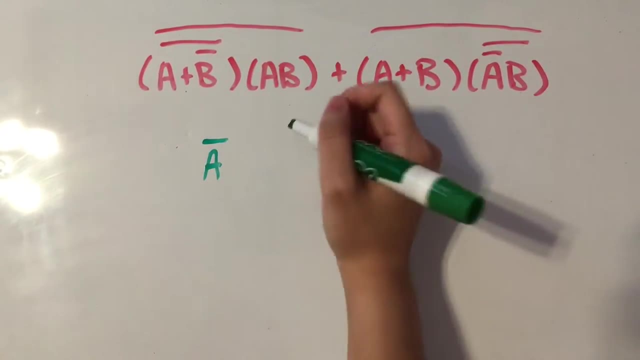 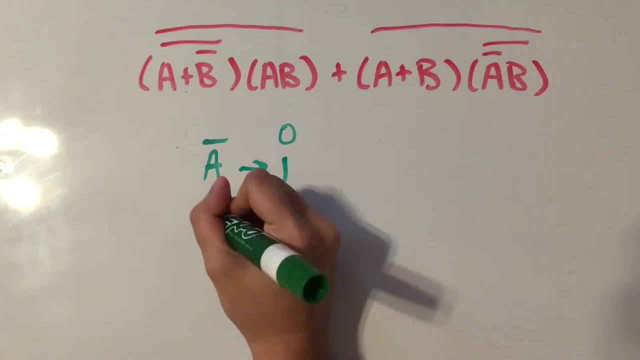 So before I go into solving this problem, let's go over some of the basics. So we have a variable a, and if we have a line over it that means not a. So if a was zero, then not a would be one. So if we have not a plus a, one of these will have to be zero and one of these will have to be one. 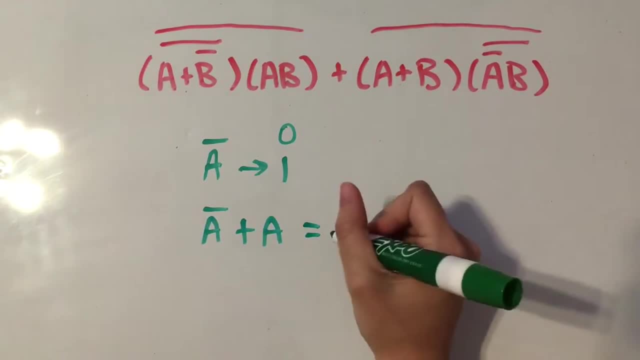 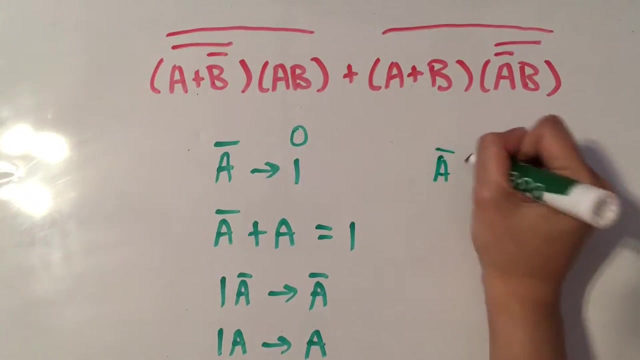 So not a plus a or any variable for that instance is going to end up as one, and if we have one times not a, that's going to equal not a, and if we have one times a, we get a. And we also have the fact that not a times a equals zero, because one of these has to equal zero and zero times anything. 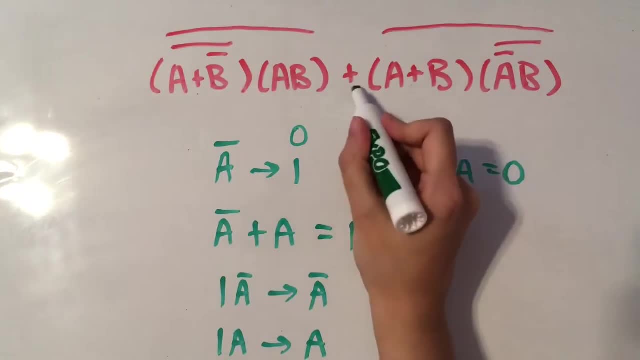 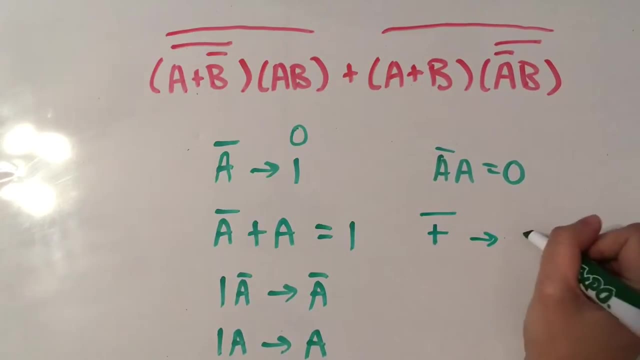 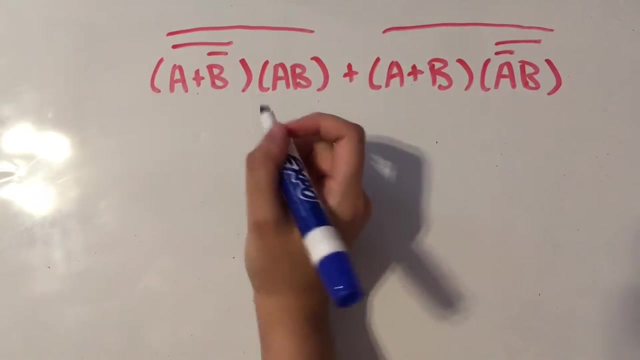 equals zero. And we also have plus and multiply. So when we have plus with a line over it which is not plus, that translates into multiplication, and same thing with multiplication: you change it into plus. So now that we know all of this, let's try to solve this equation. So let's look at the left side. first. We have a, not over all of 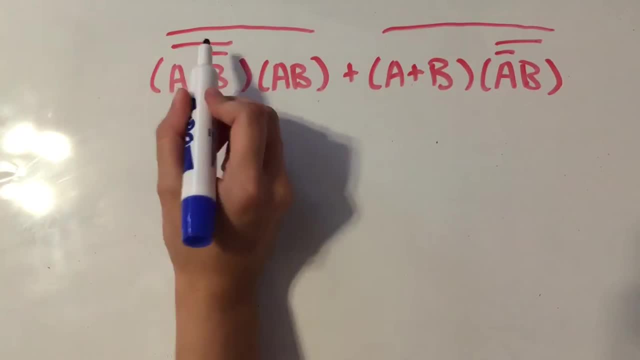 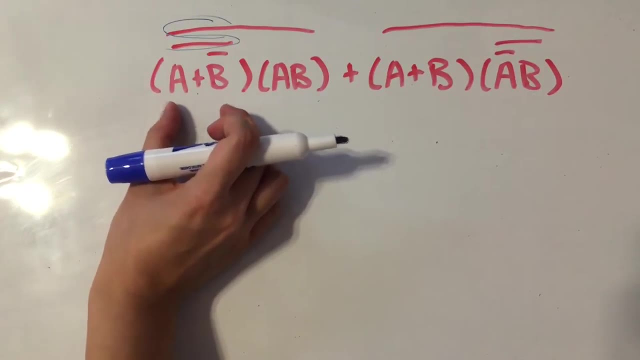 this, So these two nots cancel each other out. This one and this. So this term is not a plus. So when we have plus with a line over it which is not plus, that translates into a plus b in parentheses is basically just going to stay the same. So let's rewrite that: a plus b. 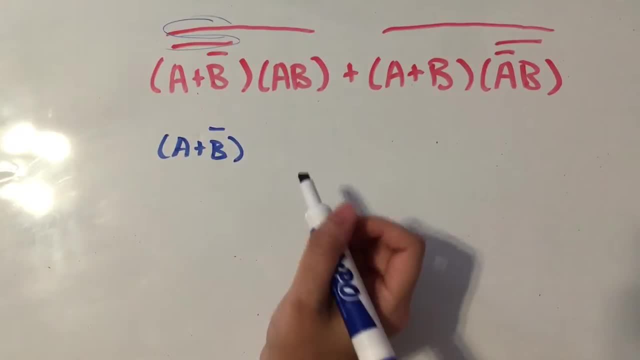 and I also see that the b has a not over it. So we also see here that the bar extends over into this term a times b in parentheses. So since we're multiplying these two terms together, remember not over a- multiplication turns into plus, So we get a plus, not b, which is this term. 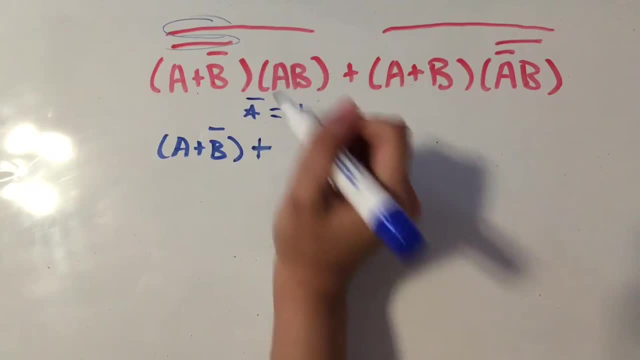 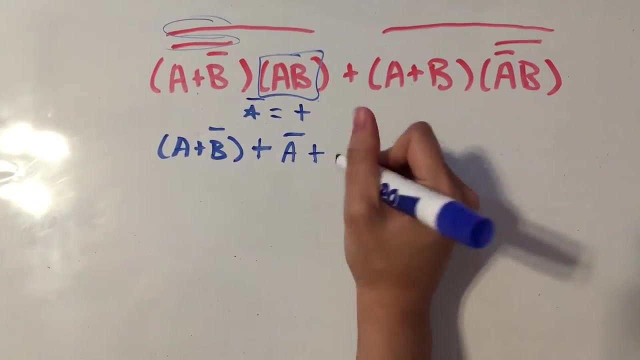 plus, since we have a not over these two And then we have the not extending over this thing. So the not would go, would distribute into the a, So a not and then a times b, So that would turn into a plus and then not b. 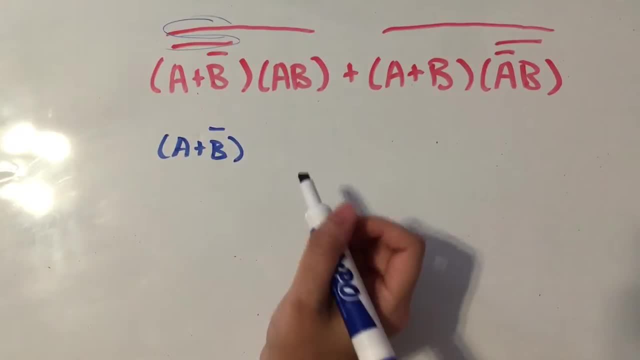 and I also see that the b has a not over it. So we also see here that the bar extends over into this term a times b in parentheses. So since we're multiplying these two terms together, remember not over a- multiplication turns into plus, So we get a plus, not b, which is this term. 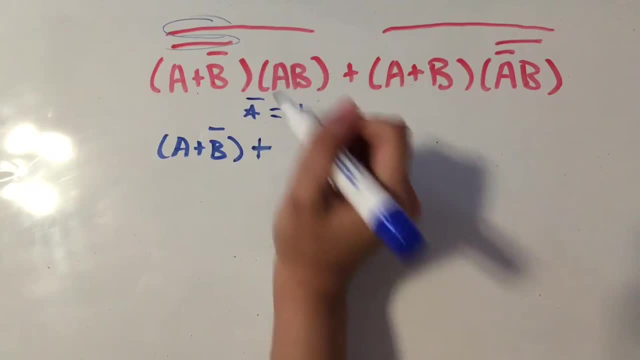 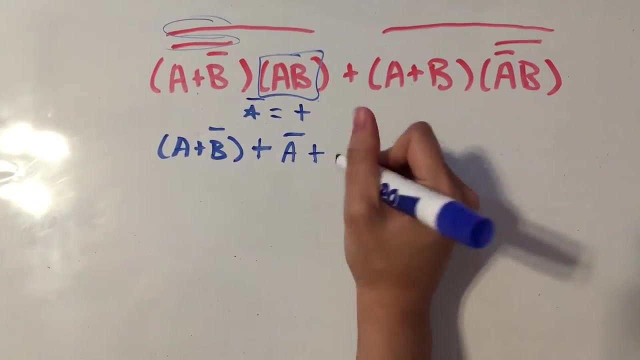 plus, since we have a not over these two And then we have the not extending over this thing. So the not would go, would distribute into the a, So a not and then a times b, So that would turn into a plus and then not b. 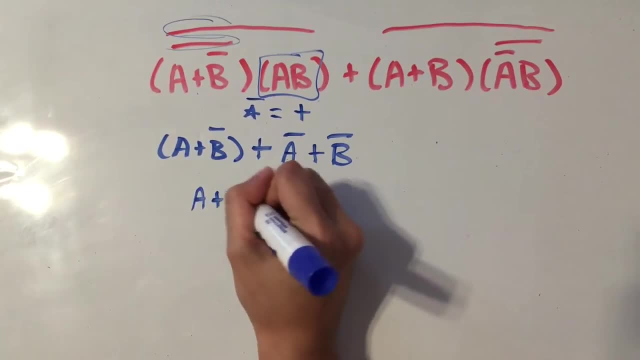 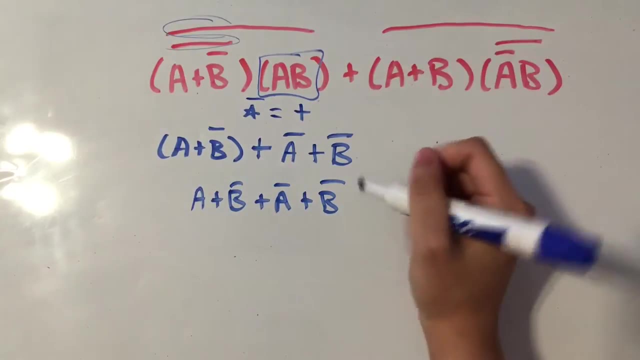 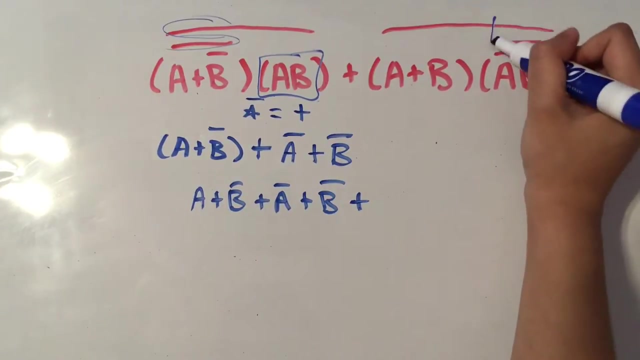 So essentially on the left side here we have a plus, not b plus, not a plus, not b. Okay, and that's for the left side. So then we have our plus sign, which we can bring down. And now for the right side, I see that these two cancel each other out. So this, not a times b, is. 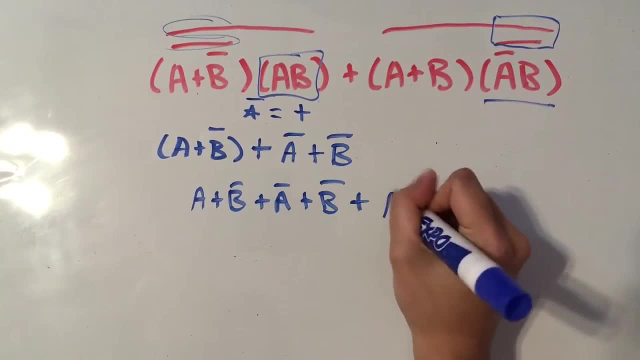 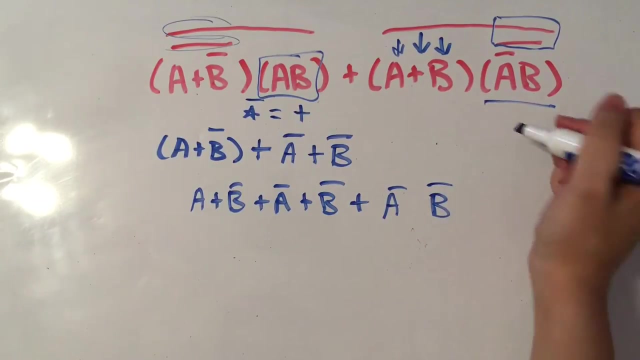 going to be left alone, And then here we'll have not a, because that not is going to come down here. The not is also going to come down to the plus sign, so that's going to be times, not b, which can also be written like this: not a, not b, And then plus because the not. 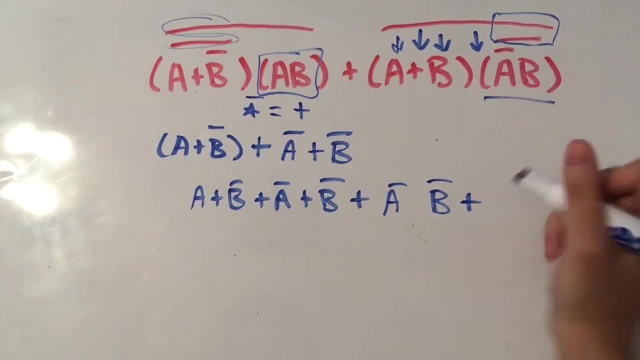 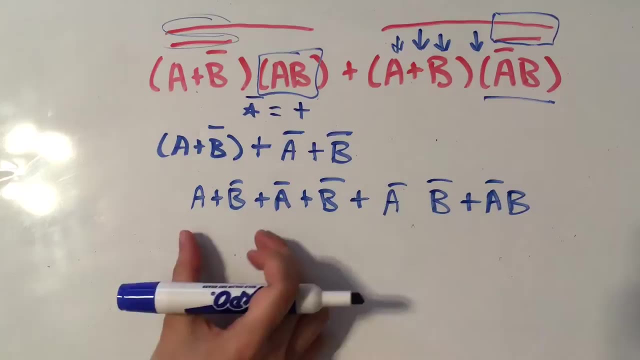 goes down there And then we have this term, which we said before is going to stay the same. So this is what we have so far, And I can see here that we have a plus, not a. So one of these has to equal zero and one of these has to equal one. So remember, we said before that a plus, not a. 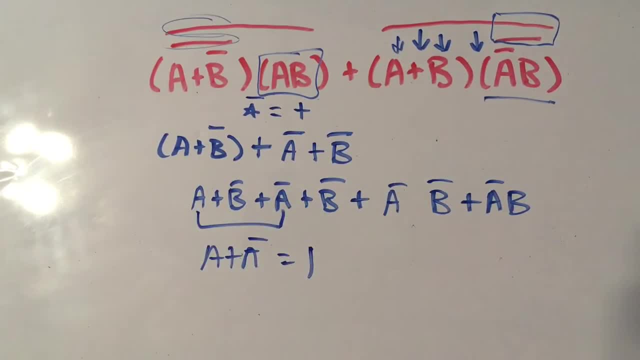 equals one, So this can be simplified to just one. And then we have these terms, Whoops, These terms left over. So that's plus, not b, plus, not b. plus, not a, not b, plus, not a b, And I can see already that this is going to equal to one, because one plus anything is just going to 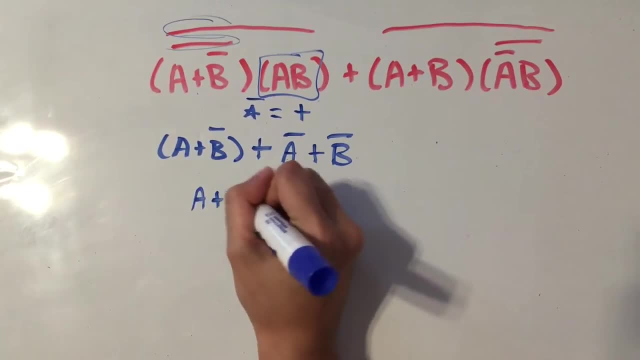 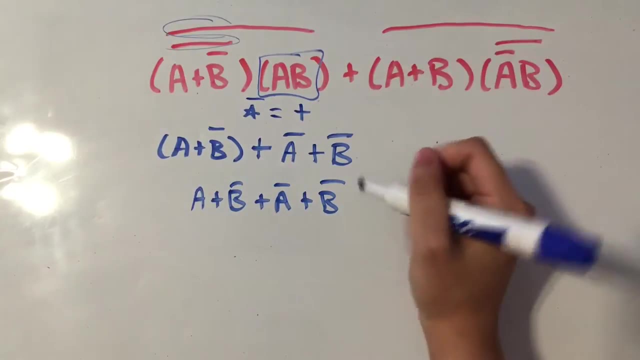 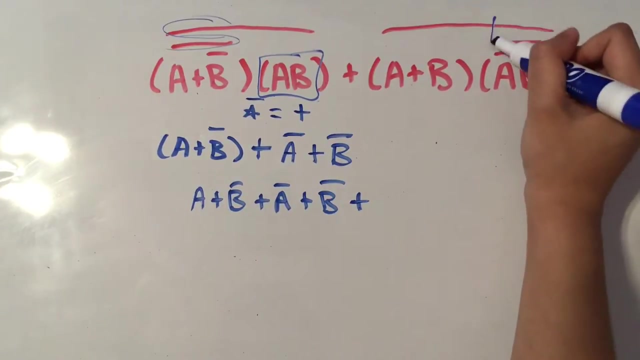 So essentially on the left side here we have a plus, not b plus, not a plus, not b. Okay, and that's for the left side. So then we have our plus sign, which we can bring down. And now for the right side, I see that these two cancel each other out. So this, not a times b, is. 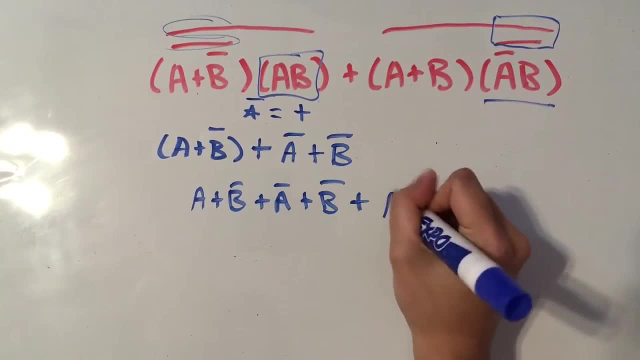 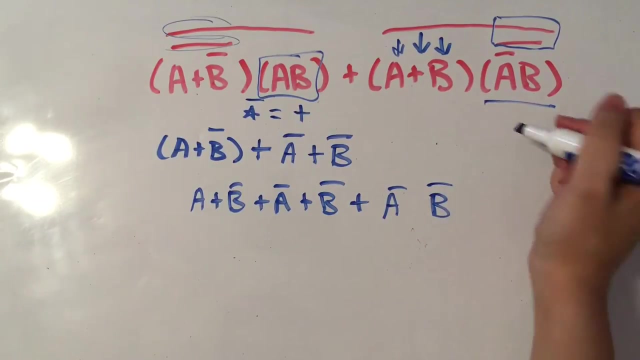 going to be left alone, And then here we'll have not a, because that not is going to come down here. The not is also going to come down to the plus sign, so that's going to be times, not b, which can also be written like this: not a, not b, And then plus because the not. 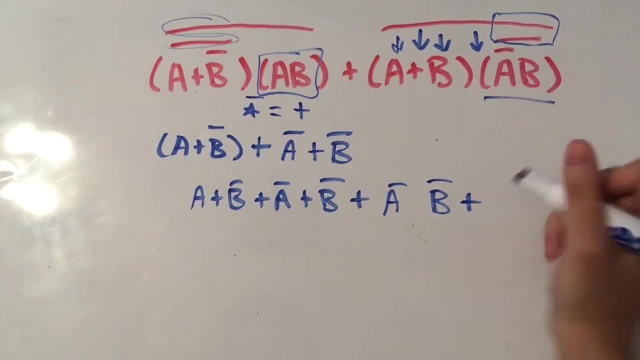 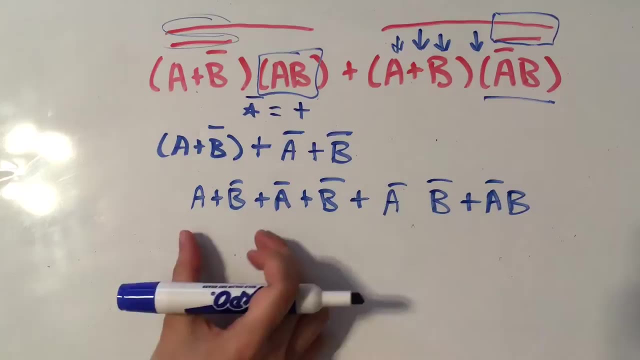 goes down there And then we have this term, which we said before is going to stay the same. So this is what we have so far, And I can see here that we have a plus, not a. So one of these has to equal zero and one of these has to equal one. So remember, we said before that a plus, not a. 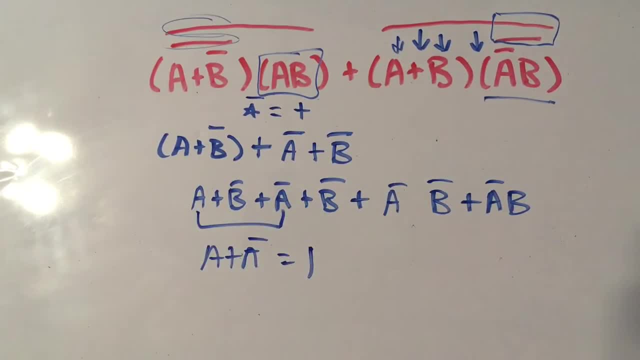 equals one, So this can be simplified to just one. And then we have these terms, Whoops, These terms left over. So that's plus, not b, plus, not b. plus, not a, not b, plus, not a b, And I can see already that this is going to equal to one, because one plus anything is just going to 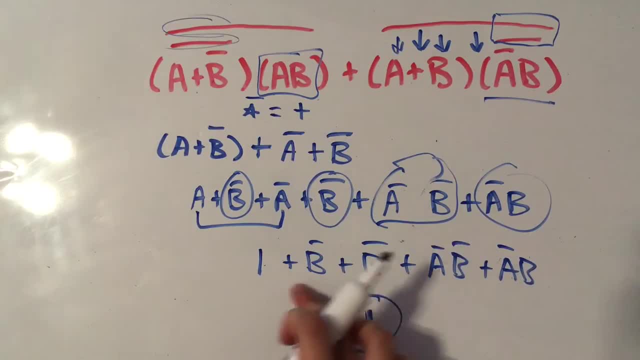 equal one, because any of these can result into zero or one. And then one plus zero equals one, And then in boolean algebra one plus one equals one as well. But we can also further simplify this, if you want to, by combining these two. So these two will just combine into not b. So one plus not b plus not a, not b plus not a b. 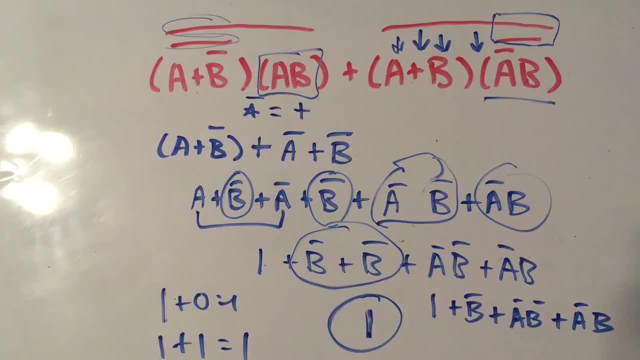 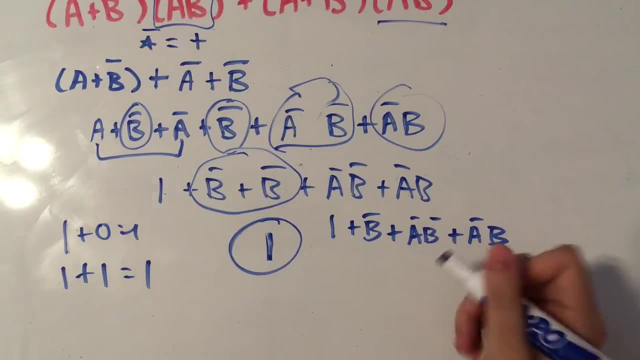 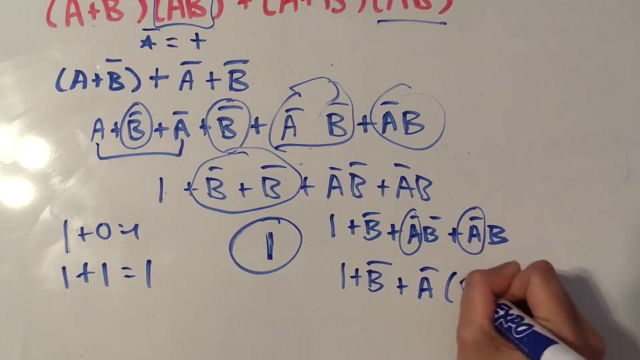 Which is just rewriting all of this here, And then you can factor out a, not a, So we'll keep this stuff by itself. So we have one plus, not b, And then we factor out the not a here. So plus not a times, not b.